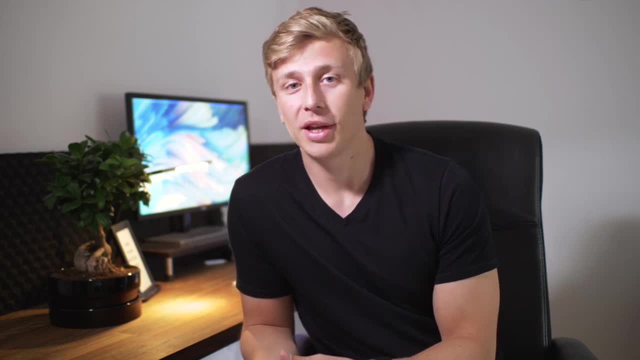 objects, And so object-oriented programming basically just means utilizing classes in your code. So if you want to write good code, then you really need to know how to use classes. So let me break this down for you. Here you see a class written in Python and that looks simple. 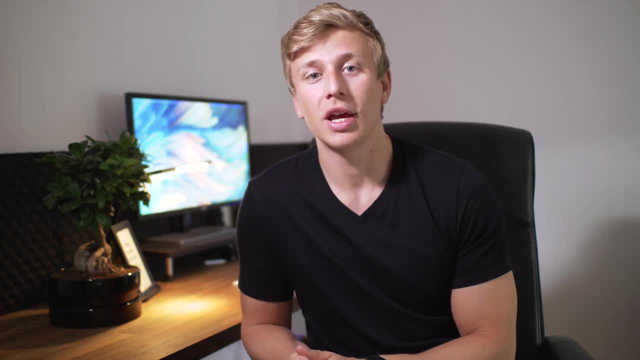 enough right, But at this point it doesn't really do anything for us. So let's make this a little bit more useful and let's add some attributes to this class, And that just means let's add some stuff that a person would have, like metrics and values, Anything that describes a person, really. 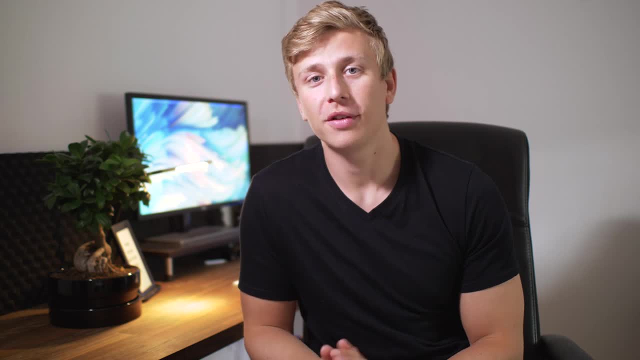 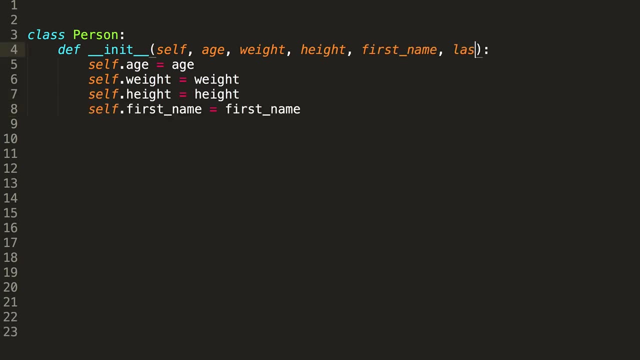 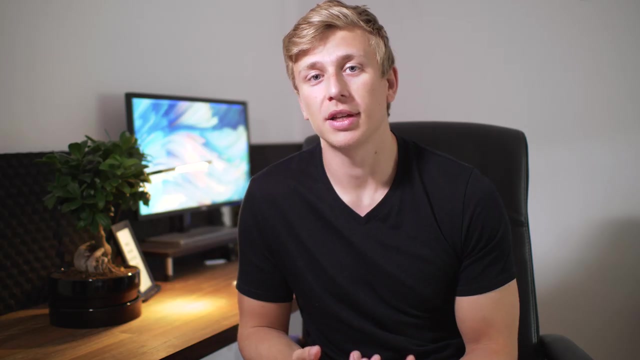 So what could this be? What kind of features does a person have? Well, they have an age right And a weight, A height And, lastly, they have a first name and a last name. So now we've added attributes to our person class and we can now start using this class in other parts of our code We can create. 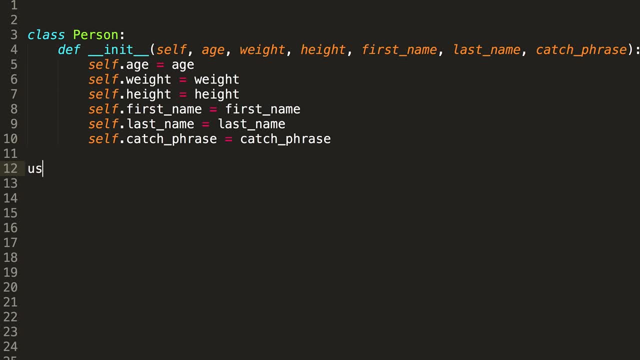 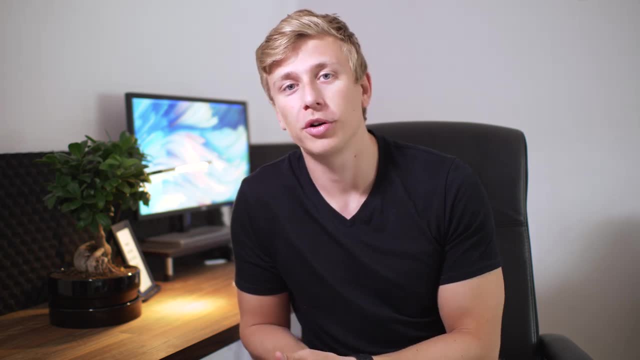 what is called an instance of our person class. We can make a new person that will be our user. let's say- And here comes the really cool part- So now we're actually able to access the attributes of person and set them for our user. So, for instance, what would the first name of our user? 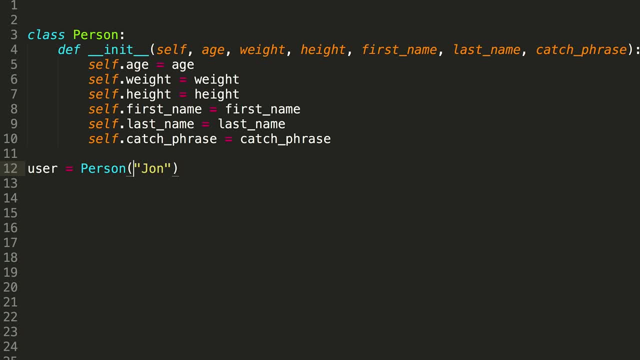 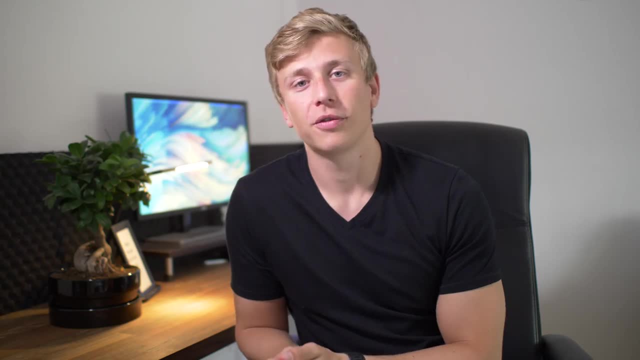 person be. Well, let's name him John. How old would John be? Well, I'm 25, so I'm just going to go with 25.. What would the weight of John be? I'm going to go with 80 for now, And this could, of course, represent: 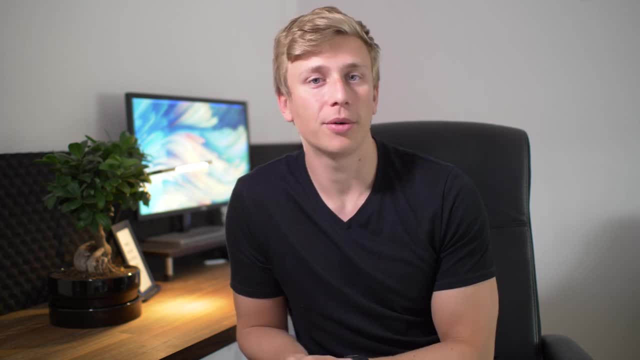 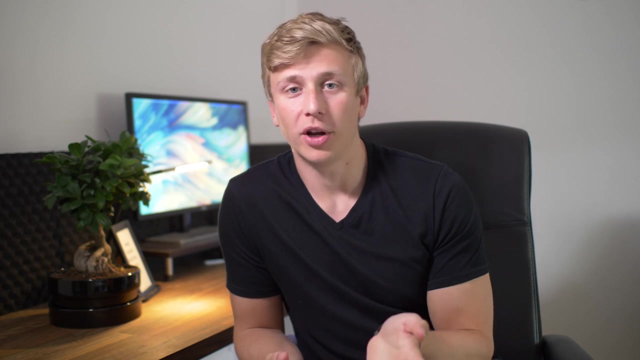 like any metric you want, So you could represent grams, pounds or kilos, It doesn't really matter. So now then, when we use our user, we will be able to access all the different attributes of our person class, And like first name, last name, age, height, weight, etc. And whatever else we might add. 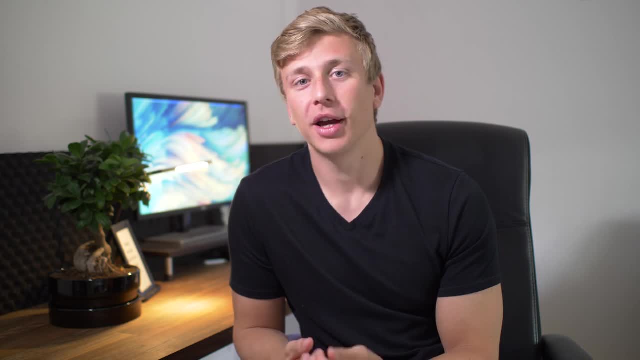 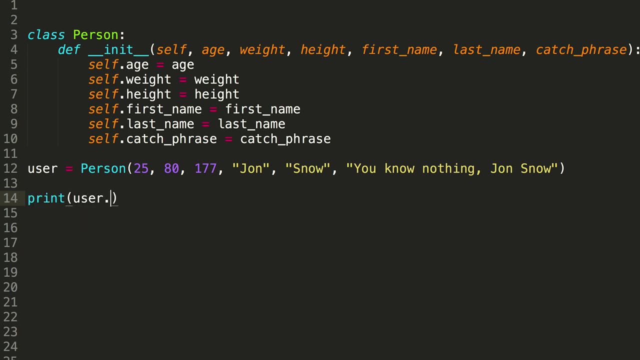 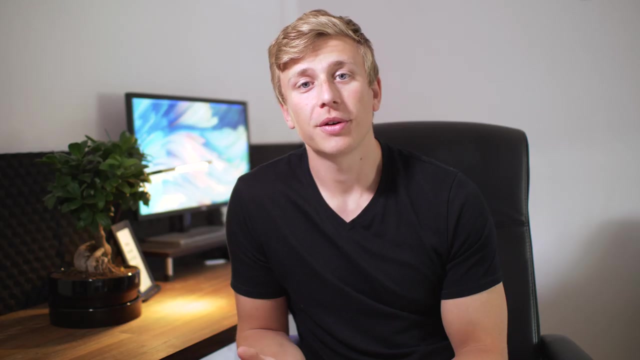 to the person class in the future. So, for instance, to test this, we could try printing the user's catchphrase to the terminal. And how we do that is just type in print and in parentheses usercatchphrase, and that will then print whatever we have set the catchphrase for our user to be. We can also add: 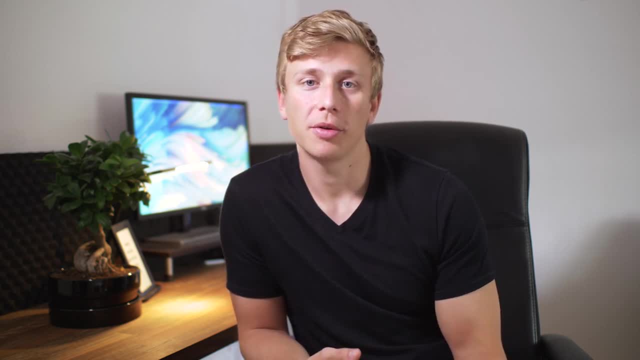 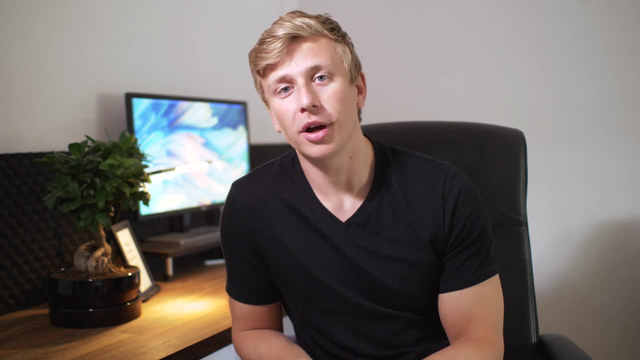 methods in our class and access them the same way that we would with attributes, And the class might then end up looking something like this: So what we can do now is we can get our user to walk, or run. Userwalk would then print walking to the terminal. You can create a class for anything.